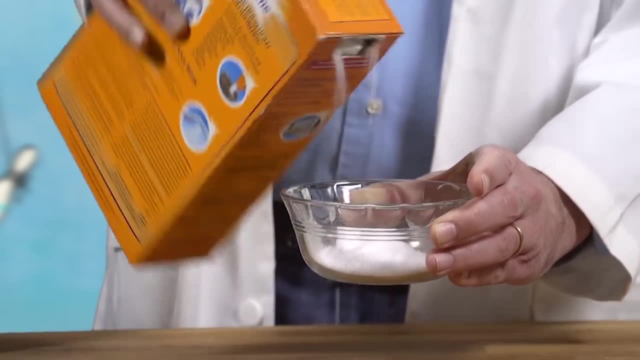 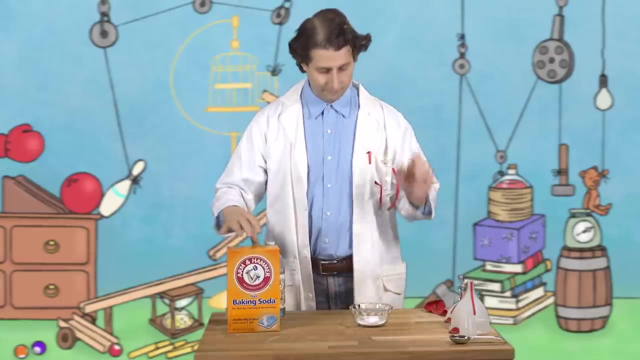 It's a white powder. You can use it to deodorize your carpets. It tastes bitter. It's useful in baking. That's why it's called baking soda. Now, what do you think happens if you mix vinegar and baking soda? 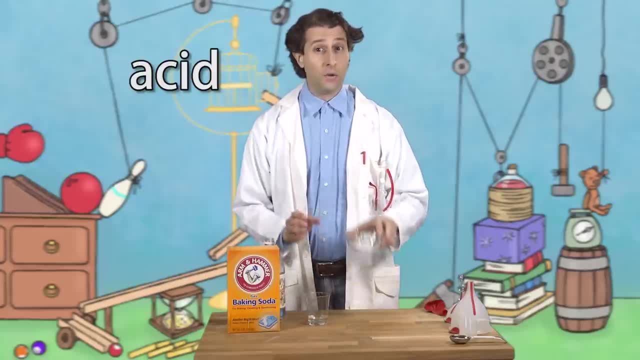 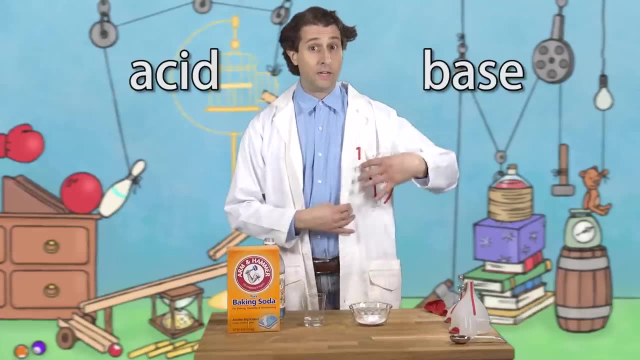 Vinegar is an acid. acetic acid, Baking soda is a base which is kind of the opposite of an acid. When you mix an acid and a base, something dramatic usually happens, so we better get prepared. Wearing my lab coat, putting on my safety goggles. 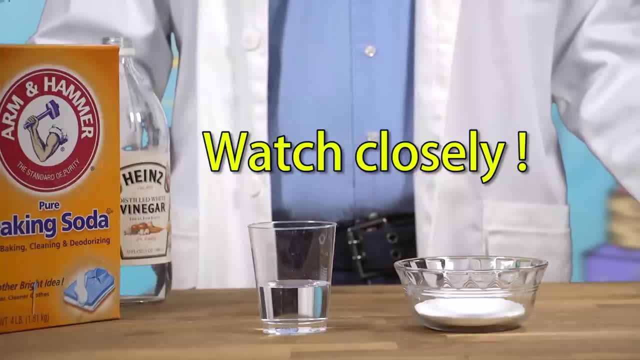 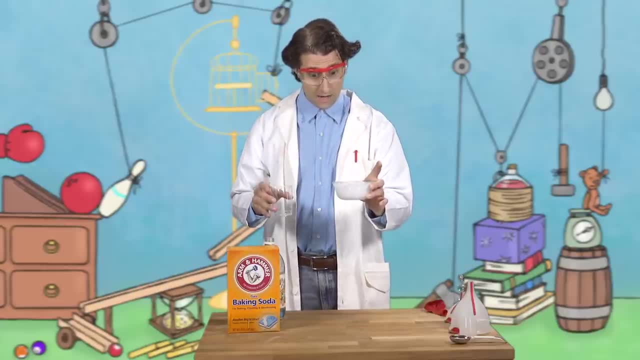 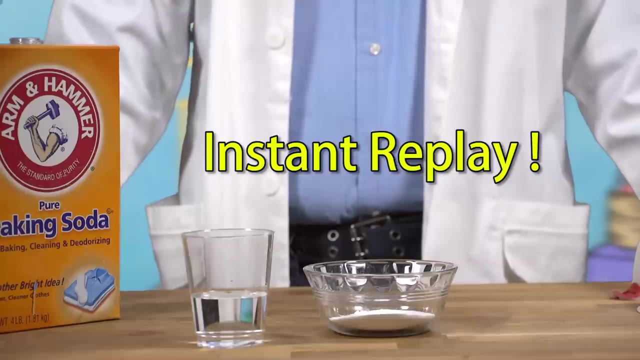 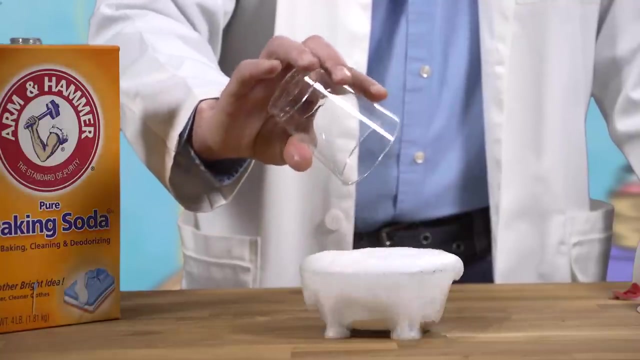 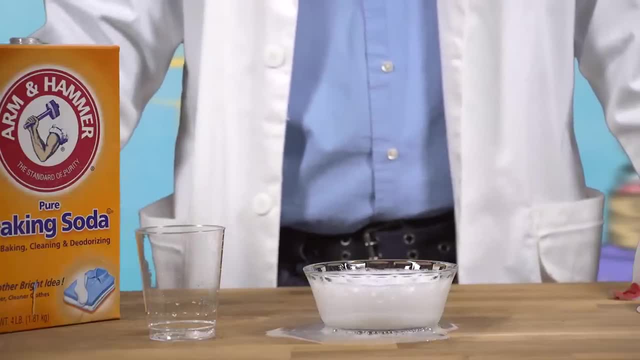 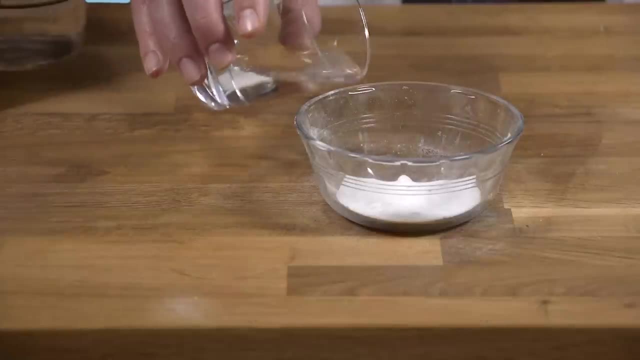 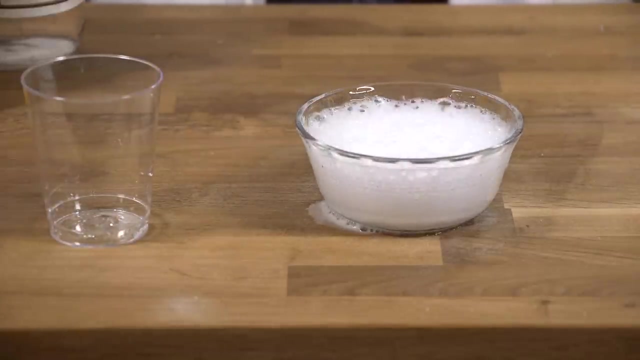 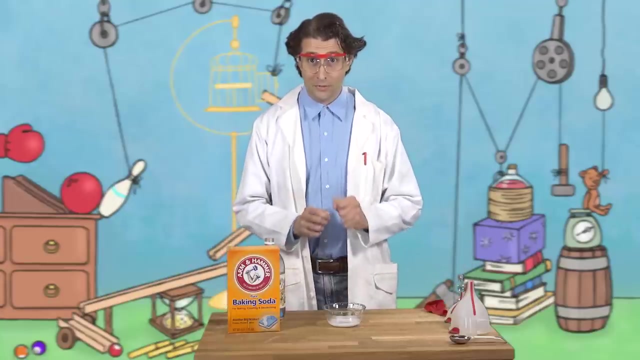 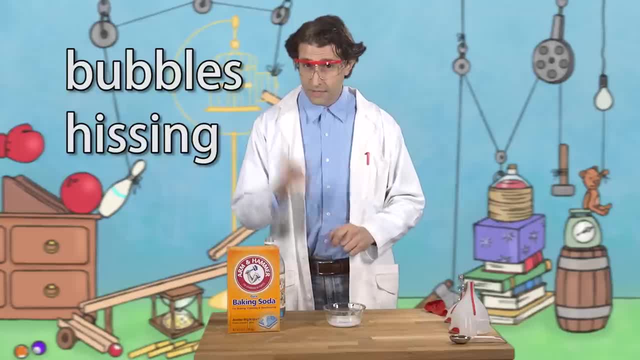 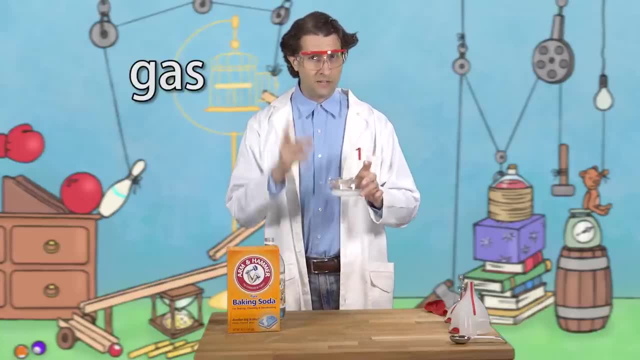 I saw bubbles. I heard hissing. What does that mean? Think, Think, think, think with your brains, Think, think, think with your brains. I think it means a gas was being released. Based on my extensive knowledge of chemistry, 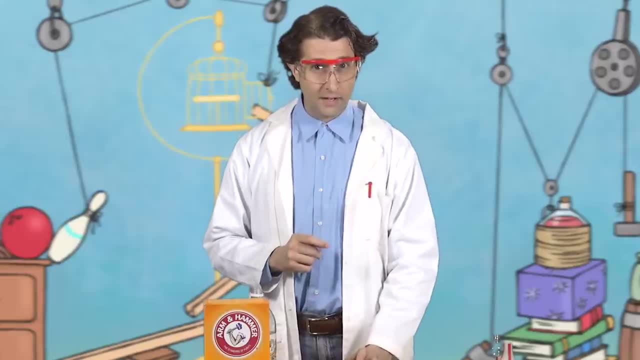 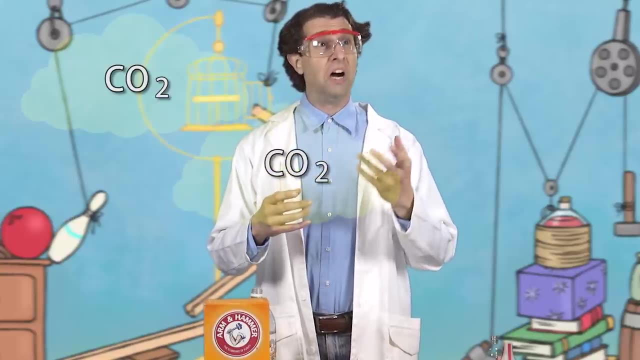 I know that it was carbon dioxide. You know carbon dioxide. We breathe it out every time we exhale Like that, And that There goes some more If I mix vinegar and baking soda together in this bottle, If I mix vinegar and baking soda together in this bottle. 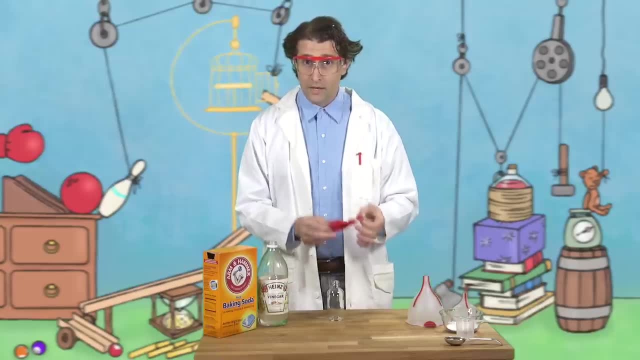 I can capture the gas being released in a balloon. I can capture the gas being released in a balloon. It may even be powerful enough to blow the balloon up. First, I'll pour a little vinegar into this bottle. First, I'll pour a little vinegar into this bottle. 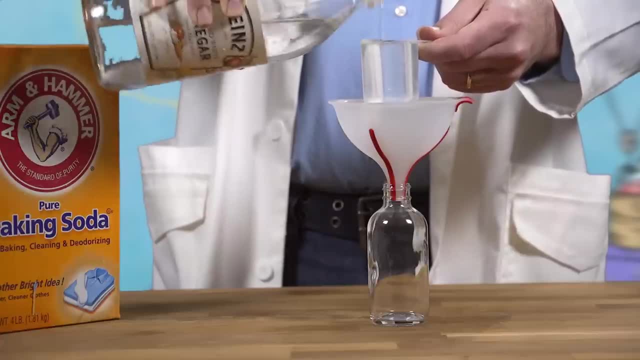 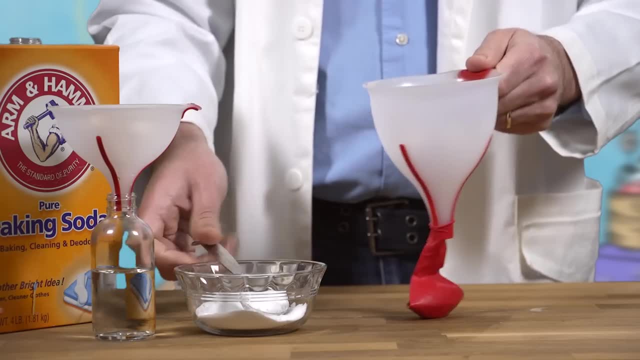 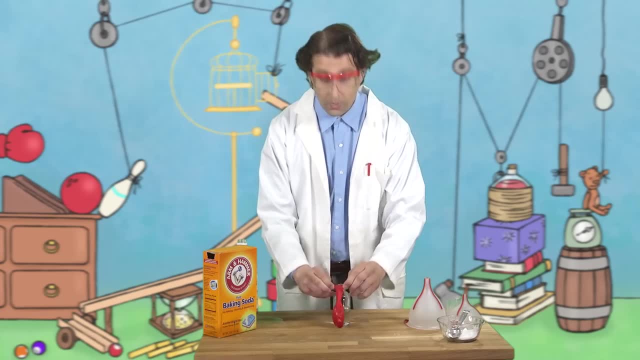 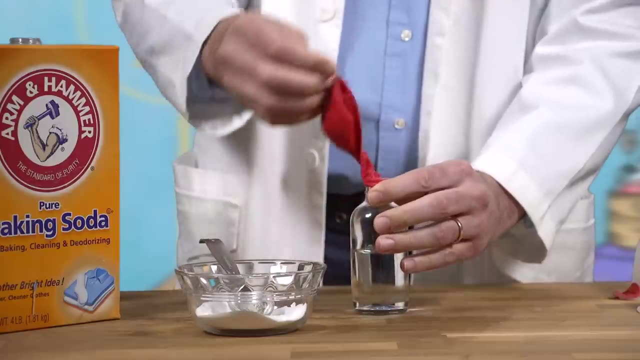 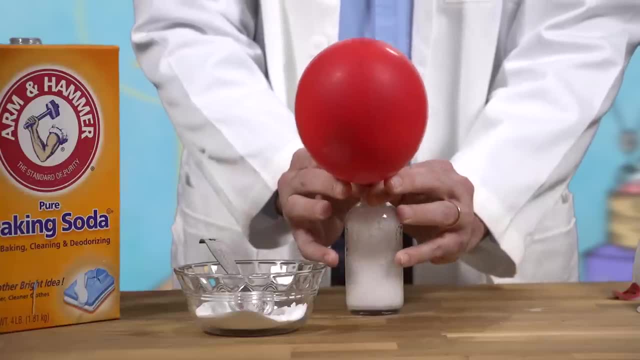 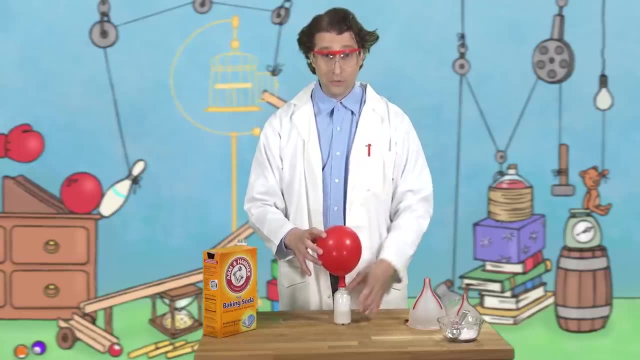 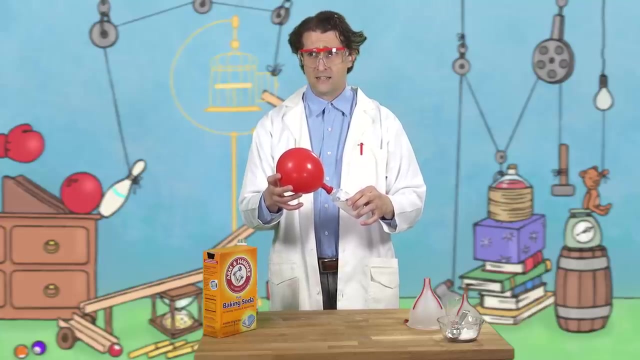 Dump in the baking soda. Lucky, here We have a balloon filled with carbon dioxide. You have a balloon filled with carbon dioxide. What do I do with a balloon filled with carbon dioxide? What do I do with a balloon filled with carbon dioxide? 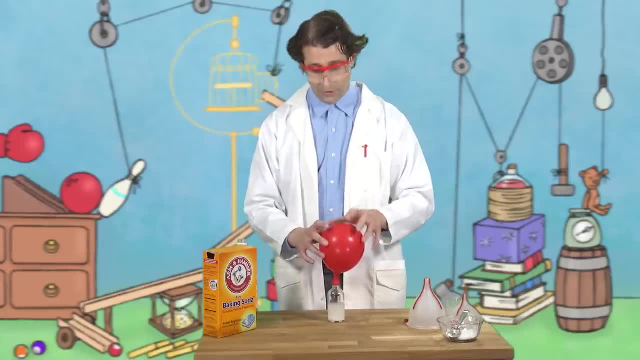 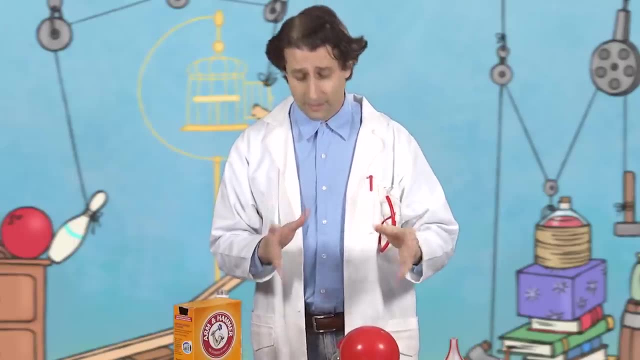 I guess we could feed it to some plants so they can do photosynthesis, But we'll talk about that another day. What do I do with a balloon filled with carbon dioxide? Some people might call it an experiment, an experiment, but it wasn't a real experiment. This was just a demonstration, An experiment. 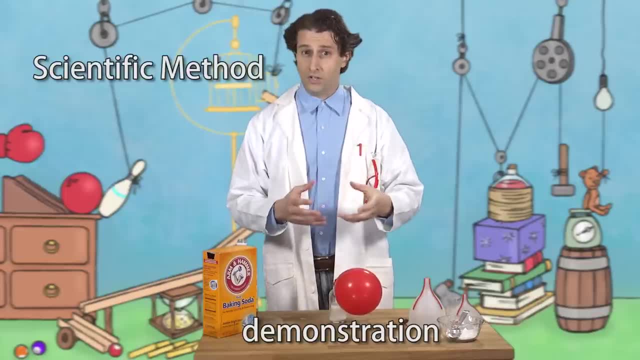 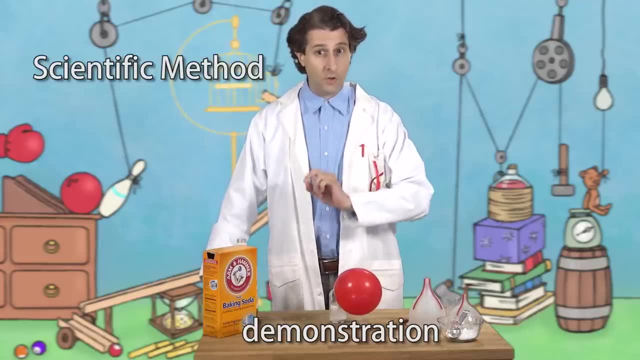 is part of the scientific method where you ask a question about how something works. you gather as much information as you can about the subject. then you try to predict the answer to your question. That is, you make a hypothesis based on what you know. 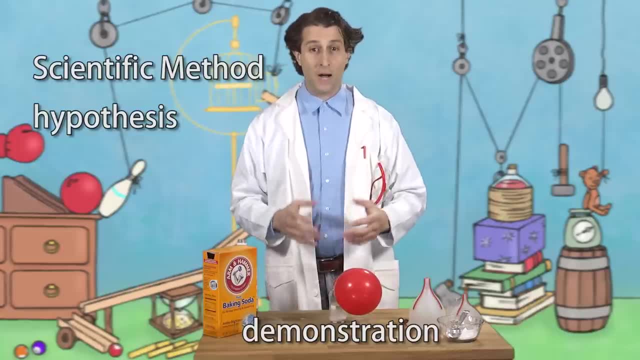 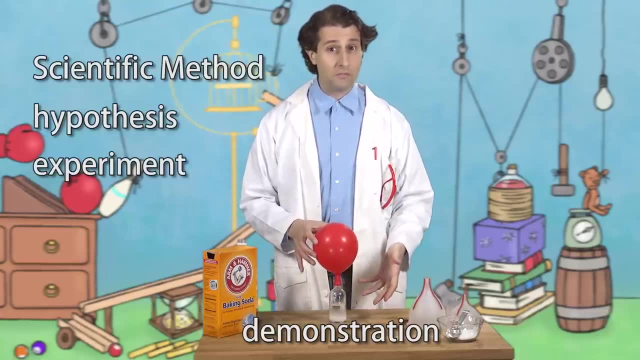 Sort of like an educated guess. Then you test to see if your hypothesis was correct. That's the experiment part. For example, what if I wanted to find out how to make more gas? Do I add more vinegar, More baking soda? Do I heat it up? What's your hypothesis Tell? 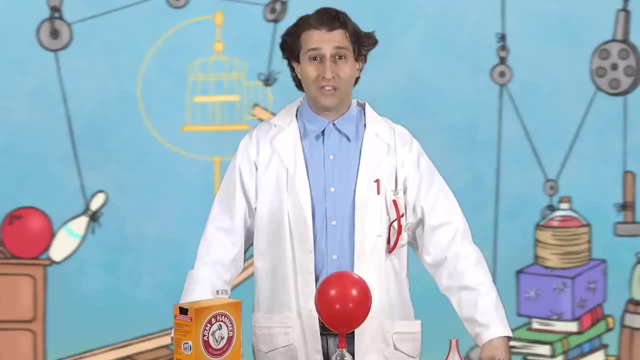 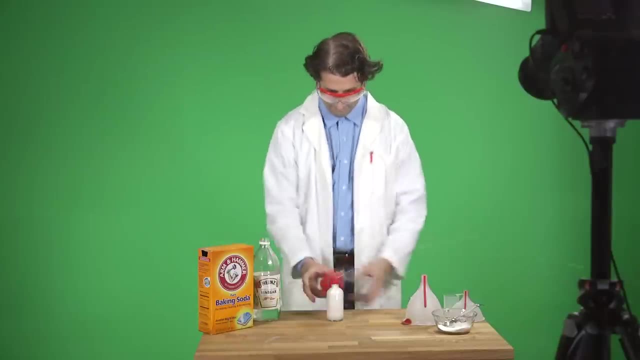 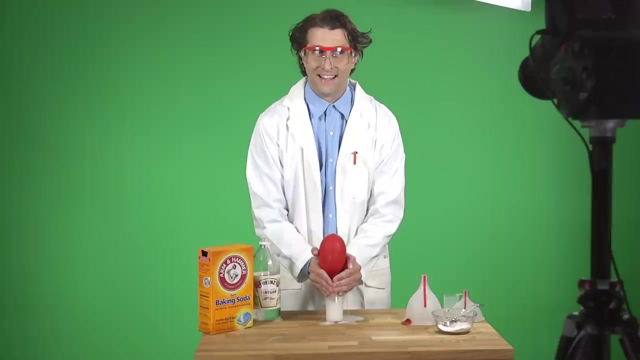 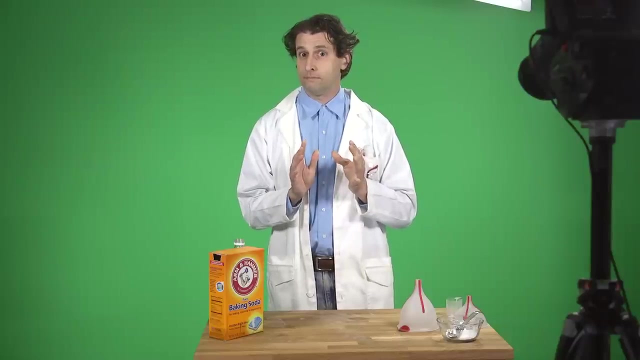 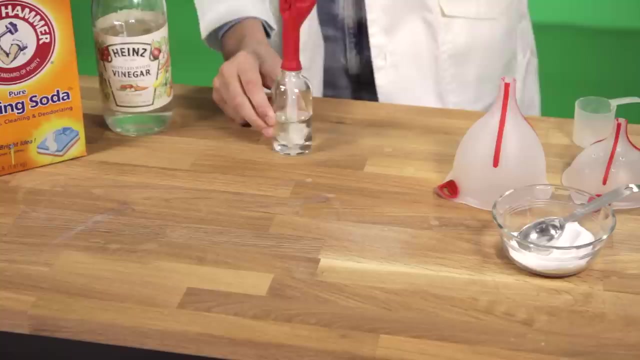 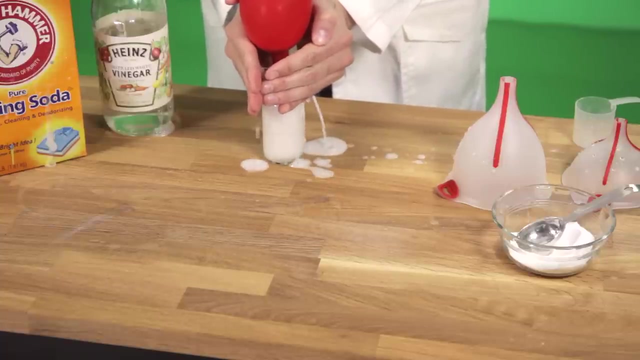 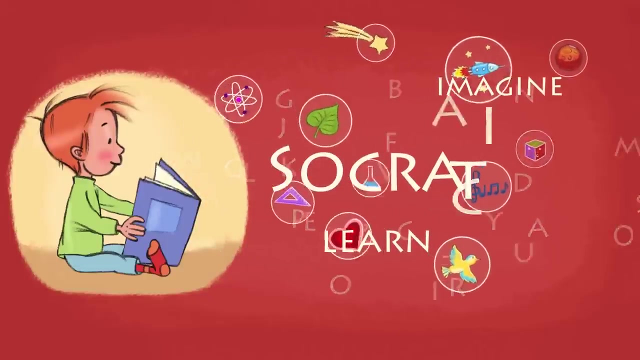 me below in the comments. Okay, that's all the time we have for science today. See you next time, Bye, bye. Captions by GetTranscribedcom. Subtitles by the Amaraorg community.